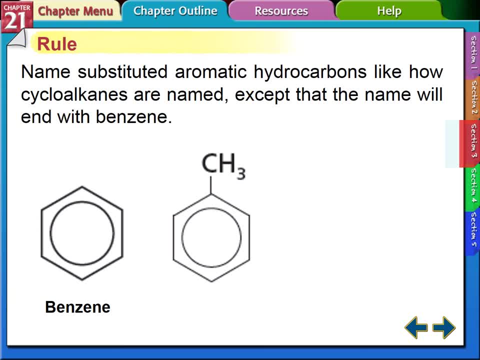 Now recall that benzene has a molecular formula of C6H6.. So if we are going to draw the hydrogen in this benzene structure, that means that each carbon atom is actually bonded to one hydrogen atom. So let me just draw that. So that's H there, Two, three, four, five, six. 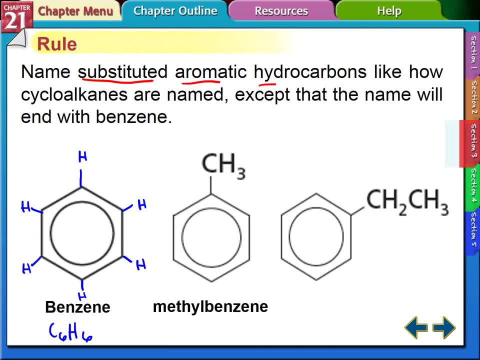 Now, when we say substituted aromatic hydrocarbons, it means that one of the hydrogen of this aromatic hydrocarbon is being substituted with an alkyl or any other substituent or others, And that's why we call them substituted aromatic hydrocarbons. 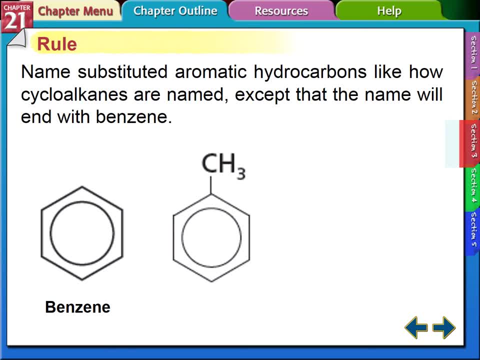 So now let us look at this example. One of the hydrogen is being substituted with a CH3H3., Which is a methyl, And therefore we call this substituted aromatic hydrocarbon as methylbenzene. On the other hand, if we have something that looks like this, the substituent is an ethyl. 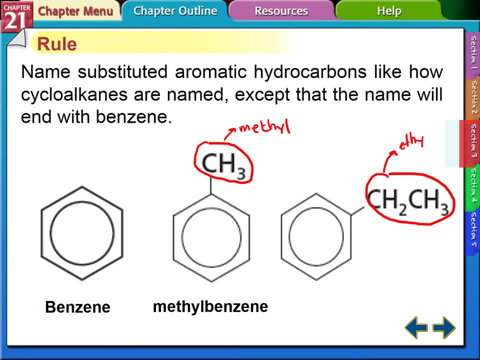 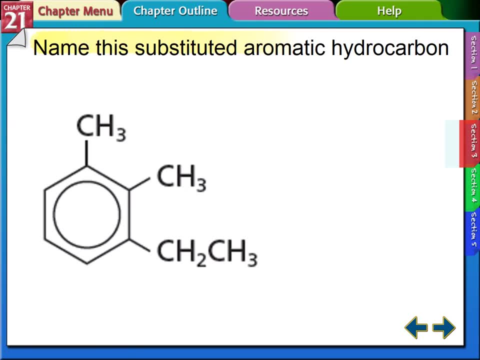 CH2CH3.. This is an ethyl, So the name of this aromatic hydrocarbon would be an ethylbenzene Name this substituted aromatic hydrocarbon. The idea is that the substituent must be associated with the lowest number possible, So we could label this carbon as one, this one two and this carbon here three. 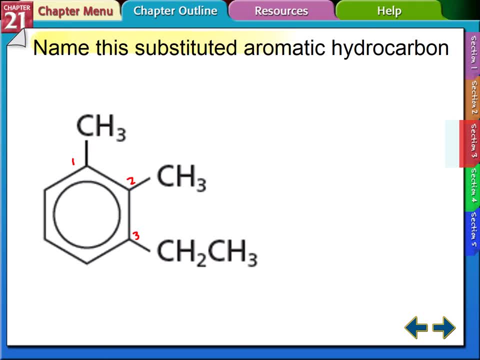 Now similar to naming cycloalkanes and any other hydrocarbons. the substituents must be arranged in alphabetical order. So this means we will have three ethyl, since the ethyl is connected to carbon. three dash one comma. two dash dimethyl, Since our two methyls are connected to. 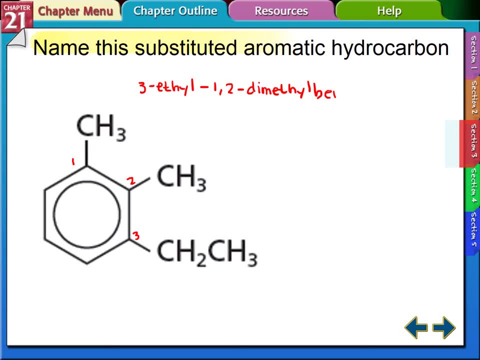 carbons. one and two, then the last name would be benzene. There is another way of numbering, of assigning the numbers to this substituent, And I will label that with blue. That's one, two and three, So with this,